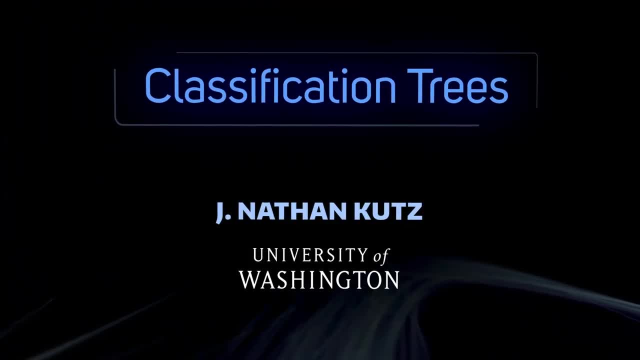 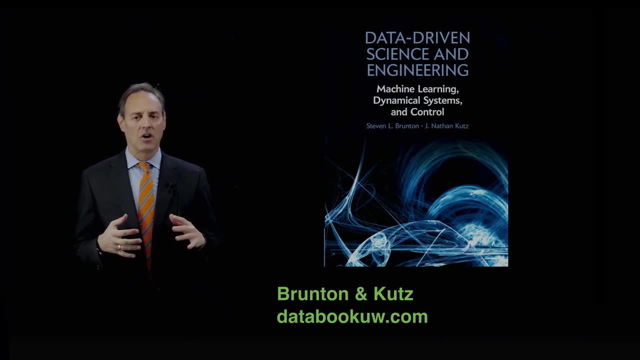 We're going to continue on with clustering and classification and talk about one of the other major methods used in practice in industry, which are classification trees. So two of the dominant paradigm algorithms used in industry for supervised learning were support vector machines, the other one being a classification tree. Both are still commonly used, partly due to their 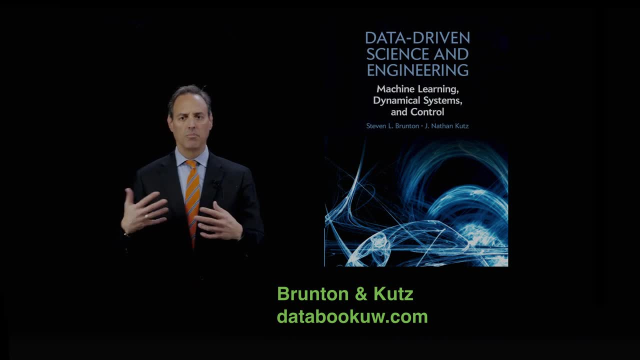 success and their flexibility, and also all the innovations you can build around them. All the details can found here at the data book uwcom, and all the lecture notes, plus code, Python, MATLAB and data. So I want to talk about classification trees and in particular, it's. 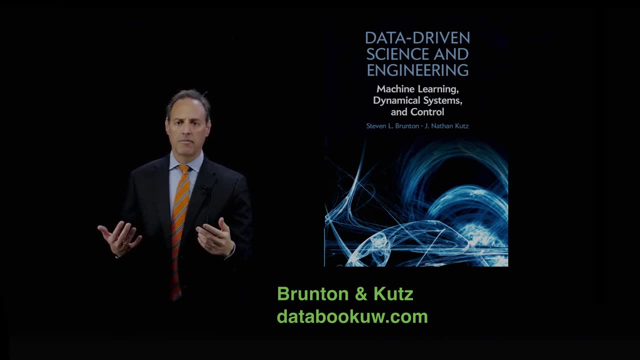 it's an algorithm that's very straightforward to use. It's you're not solving some big optimization problem. You are scanning through your data, and so that that is part of the cost of these. but it's a very effective tool, and I'm going to just tell you how. 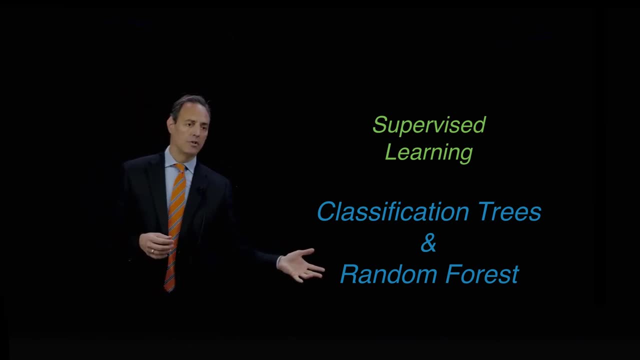 it works, And also there's versions of it called random forest that I want to highlight, which is one of the important uses of it, especially as you. what you would like to do is build ensembles of these trees Every time you split the data from a training sets, unique to that training set. but 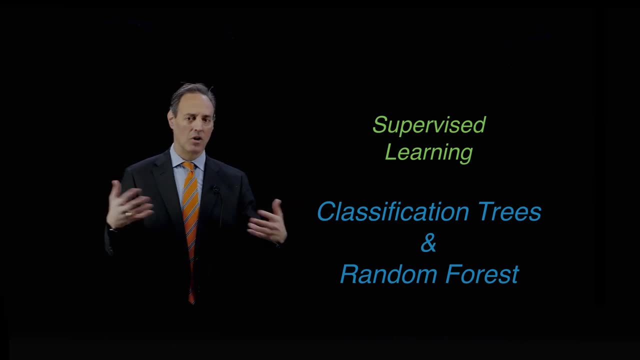 you know, just like cross a validation, would you do it over several draws of that data. you would get very different results and so you would not very different results. but especially as you start splitting it would be different. but then you would maybe average over those to do a random forest and 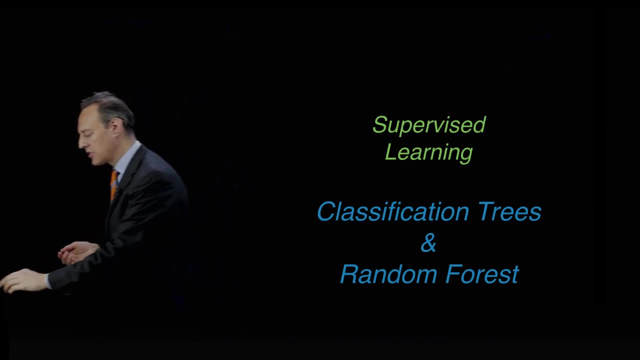 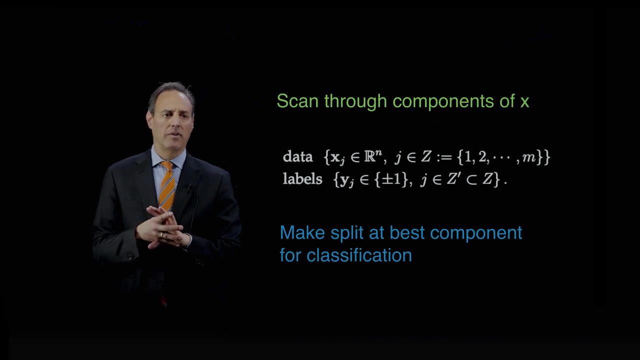 build an ensemble of models. Okay, so how does this work? It's actually pretty simple, So let's go back to the setup about supervised learning. What I give you in supervised learning is data and labels, right, so the data set are some n-dimensional vectors which are the features of the measurements. 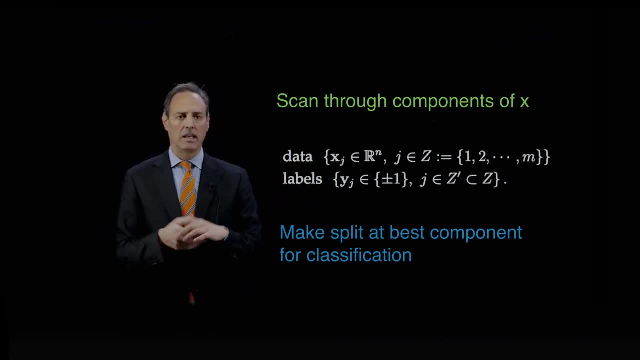 you collect out of the system and there's, let's say, m points and each one of the points has n features and each one has a label plus one, minus one. So what we're going to do is we're going to take this vector. so the x of j here, reminds me, represents the jth data point, which has n. 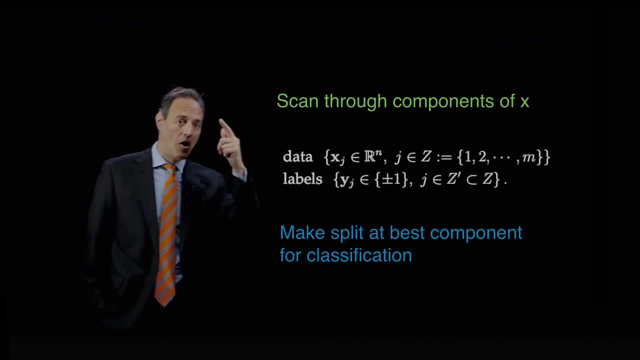 components and what we're going to do is we're going to scan through all n of its components Across the entire data set. so I'm going to say component one of the vector. let's look at that and let's actually look. if I just look at component one and I just try to associate component one with 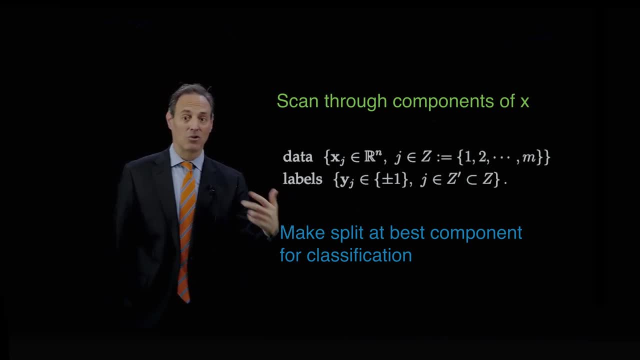 the label being plus one or minus. well, how well do I do? Okay, so if I just use that component to make a classification decision, how well do I do? and I do it for all n components, and so what I do is, as I scan through each component, 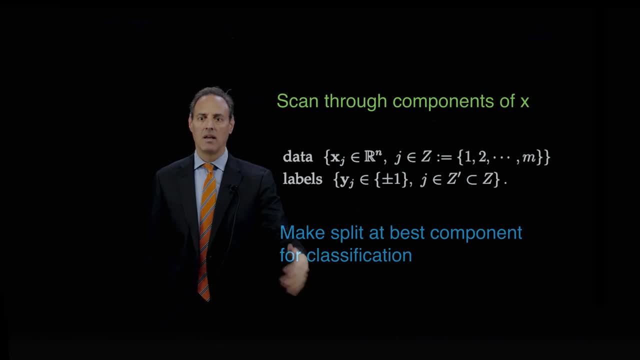 I look at the one that did the best in classification of the data by itself, The one that did the best. that's where I design a split, in other words, in the second component print, for instance. for instance, here could be that if I look along the second component, it's: 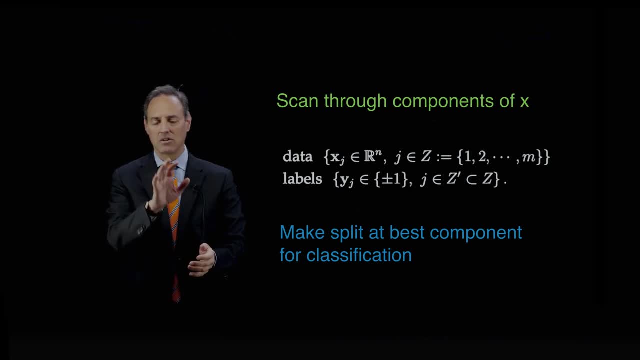 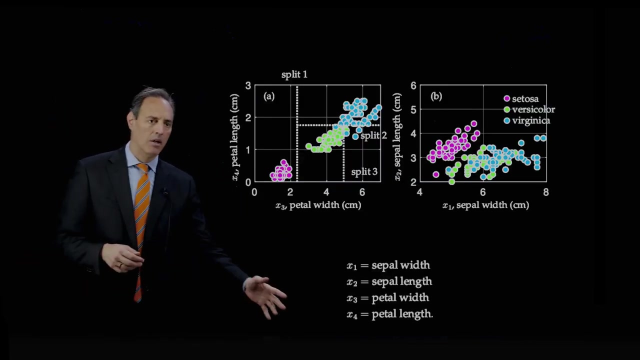 it's a very good division of dogs versus cats, so you would split right there. that's your first tree cut, or first branch that happens in your decision making process. So let me show you a simple example of this, and this is the iris data set that we've played along with before. so we have 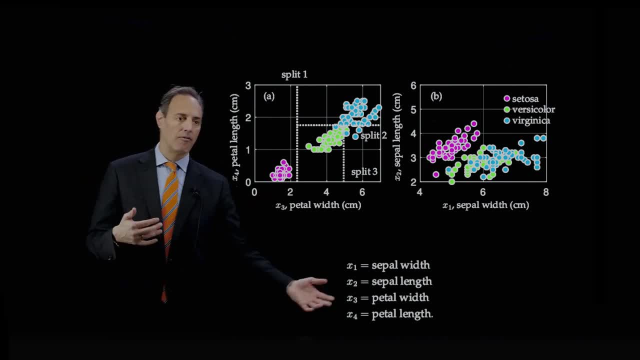 four features: the, the feature space. the measurements are four dimensional: the sepal width, sepal length, pedal width, pedal length. there they are x1 through x4. so we have these four features, we have the measurements across the data set. we also have up to three labels. right, we have satosa versus color. 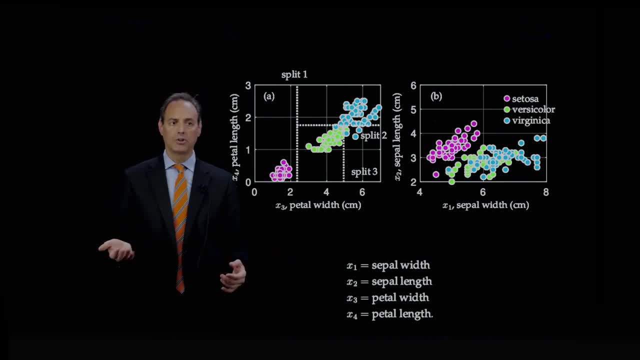 virginica. those are the three labels we have for this. so what you're going to do first is walk along the x1 direction, and so what i've drawn up here- this is what you're seeing over here- is x1, x2, x3, x4, and what i'm 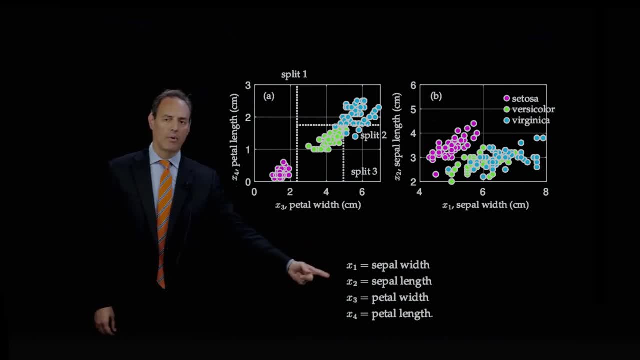 going to do is do mental exercise. let's go along the x1 direction and see how well does splitting in the x1 direction do in terms of separating the data. so here's the x 1 direction. if I walk along here, notice it's very hard for me to cut anywhere in the area I'm going to cut into ay. 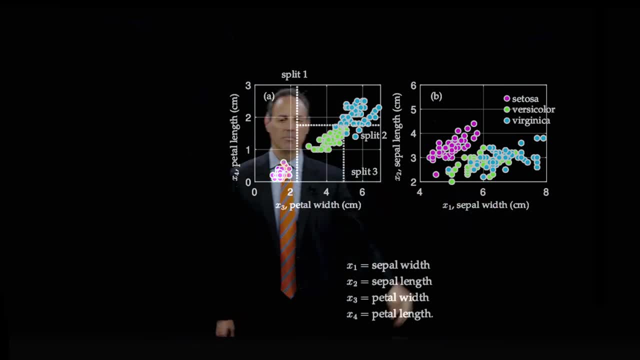 in the X1 direction and get a very clear discrimination between the magenta, green and blue balls. What about the X2 direction? Come over here, scan in this direction and again you see pretty hard to draw a line here that separates the magenta, green and blue balls. 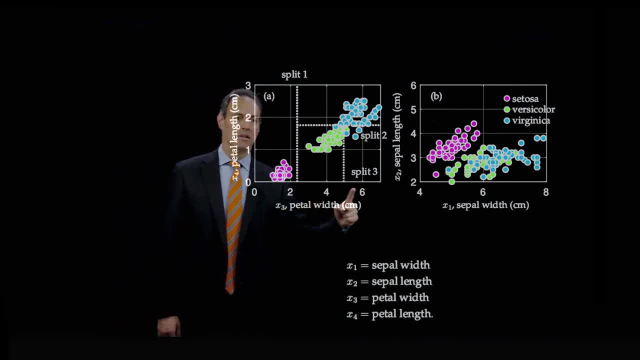 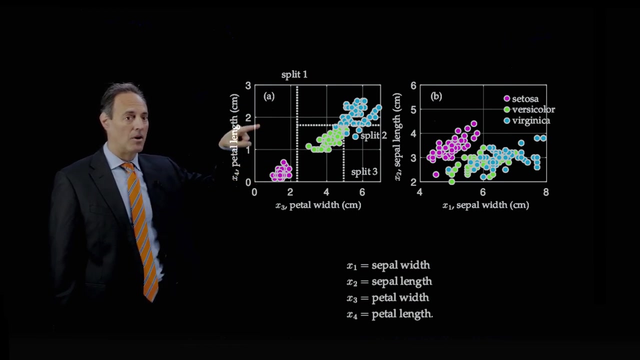 That's about the X3 direction. If I scan along here, this is quite remarkable because in fact I can completely separate the magenta balls from the rest of the data. So the X3 direction looks very promising. right, And in the X4 direction again, I can scan this way. it also looks pretty promising. 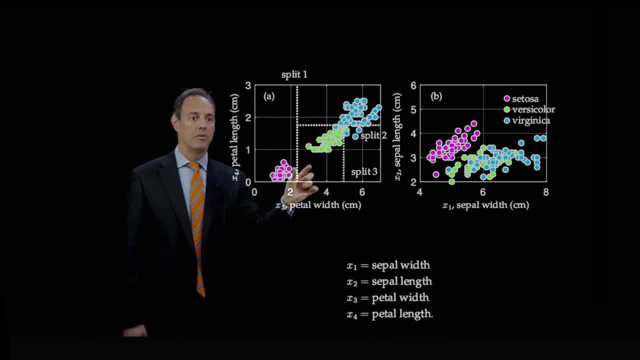 although it doesn't look quite as- look at, the gap here in the X3 direction is a little bit bigger than the gap in the X1 direction. Okay, gap here in the X4 direction. So what it decides it says, I will split here along. my first split. 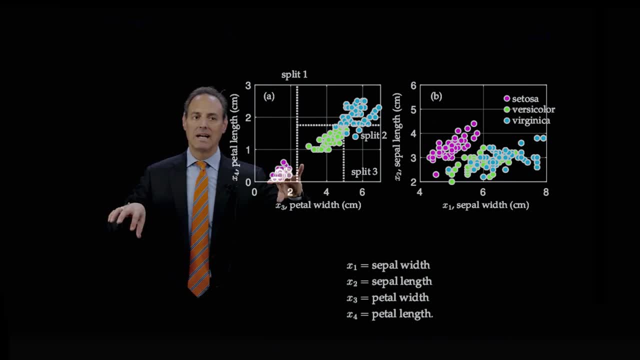 is in the X3 variable, I get a very nice separation between this class of magenta balls and the rest of the data. Okay, that's your first split. You've made a decision. Now the way the splitting works is now. you've said: okay, now I can take this data out of the picture, because now I've basically 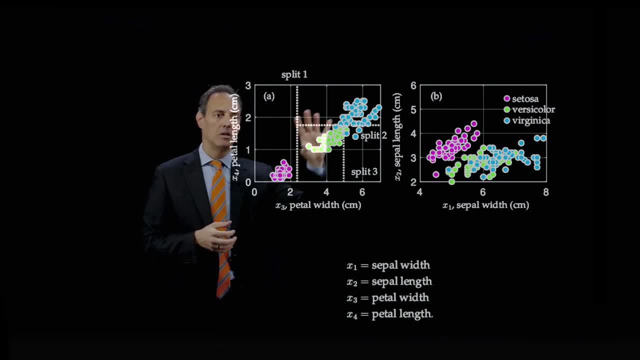 said: okay, so I've got the split here. Now let's look to see what's going on over here with the rest of the data. Now let's go to a second split. Again, I can scan through the data and say which direction. 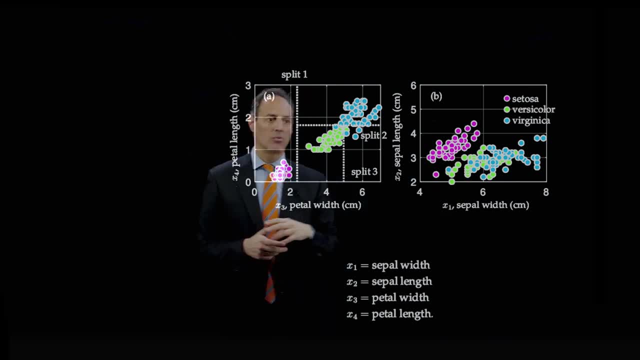 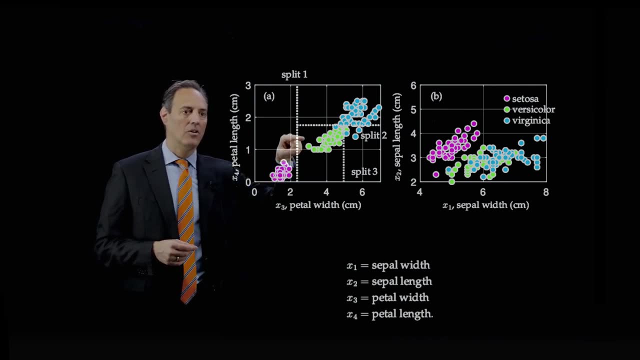 gives me the best split. Again, I can look in these directions: The X1 and X2 don't give me much, but as I scan along the X3 direction- or sorry, the X4 direction here, notice, if I go this way I get a. 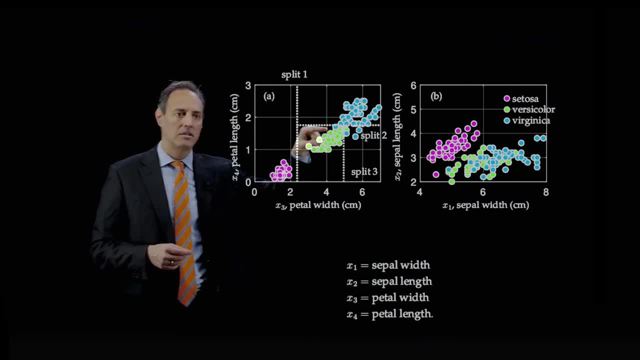 pretty nice split between the blue and the greens. So it makes a second split here. Now you walk along X3, split again, So you can split along a variable direction multiple times. but at each iteration step you go down a branch now and you scan across the variables, decide if you're 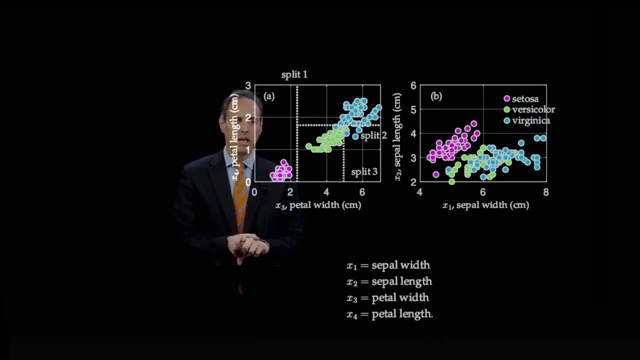 going to split again and again, and again. Okay, Now, how many times you split? Well, that depends a bit on how many labels you have. Okay, So here what we know is we have three labels, So we have three types of. 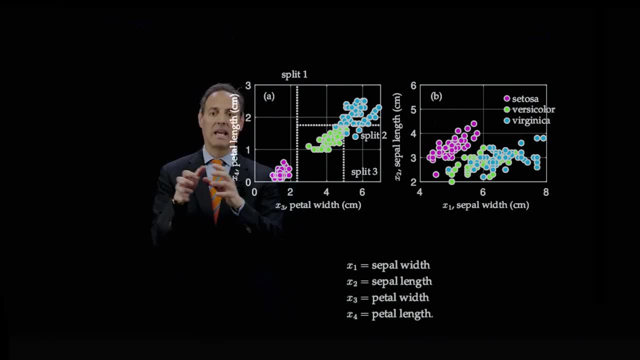 flowers, and so I'm going to do three splits to try to see can I split in these feature directions in such a way that I give you the best discrimination between the three clusters of viruses. Okay, And so this is a nice picture because graphically you can see what the process is And also that I'm just scanning through the. 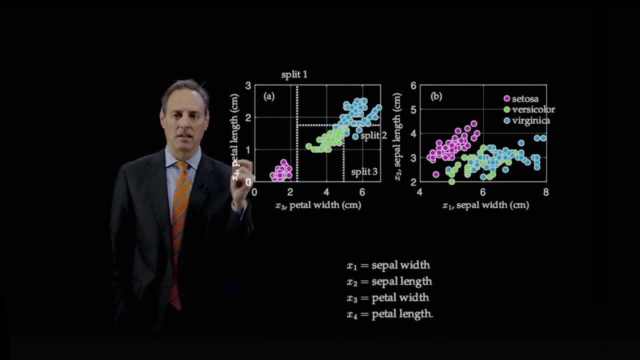 data. The algorithm is a very simple: scan through the data And there's an if statement and four loops. So no high-end optimization here, Just scan through data, which can be costly if it's very high dimensional, but it gives you a nice way to go about supervised. 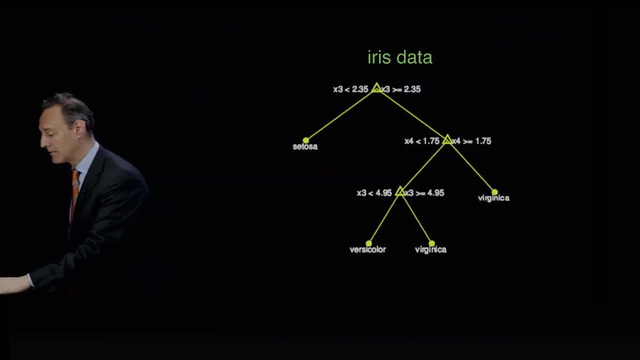 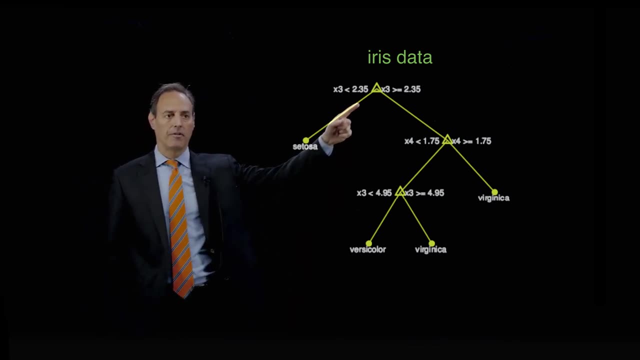 splitting of the algorithm and generating a tree. In fact, for that iris data, here's what these trees look like. Okay, So, first of all, your first split was right here: X3, less than 2.35 or greater than 2.35.. 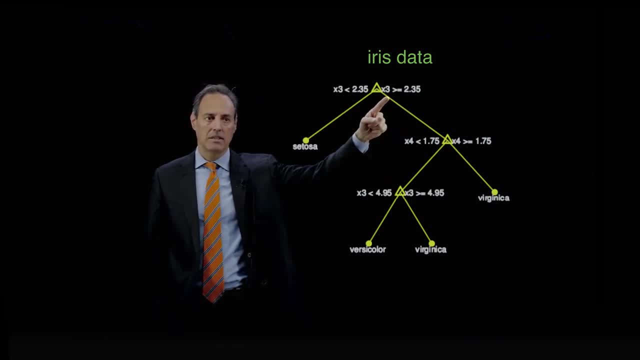 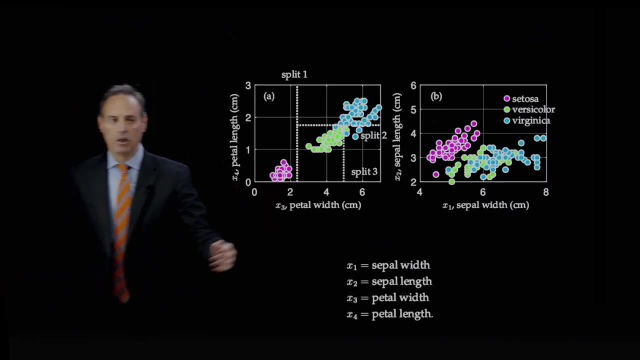 Greater than or equal to 2.35.. If it's less than 2.35, I'm labeling those setosas. Okay, In fact, let's go back here. look at the value here. The value right there is 2.35.. Okay, That's. if you run the code, you'll find. 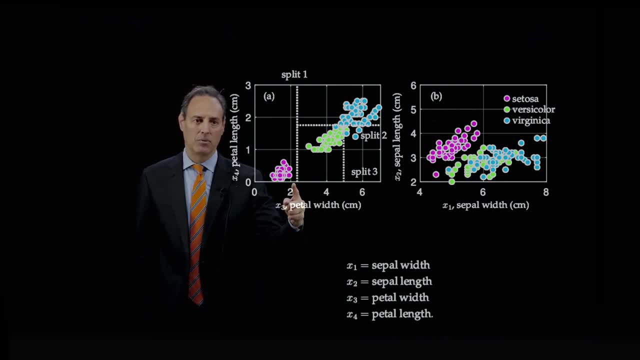 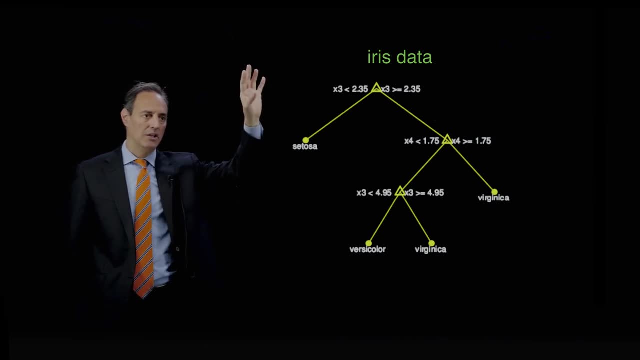 that split, You'll find that this here is the best separation point: 0.235.. So that's what the first split was, And over here is setosa, and then you just leave everything else down this bracket. That's what I'm. 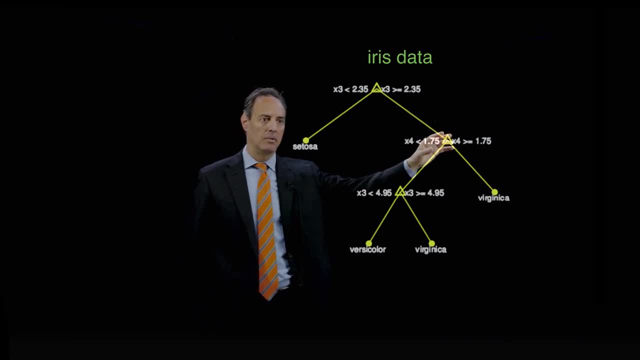 branch over here. So now you come down this branch. Now you have your second split. X4 is less than 1.75, greater than 1.75.. Okay, So that was this split right here. Now we're not quite ready to. 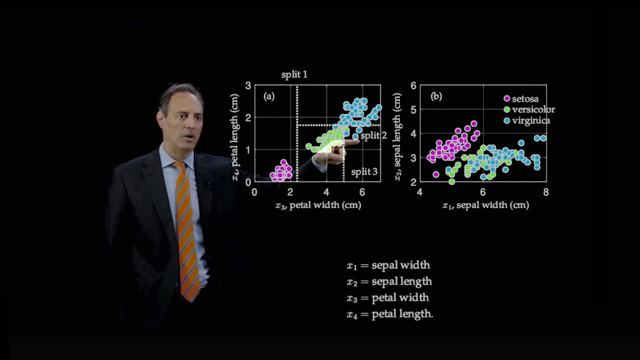 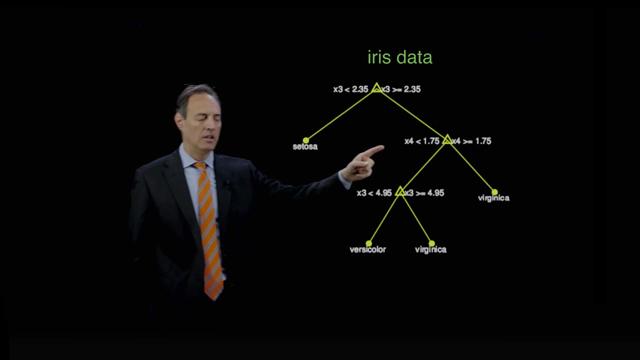 classify yet because, notice, when we do a third split, these blue balls are going to be part of these blue balls. So the blue balls are going to be part of these two pieces here. The green is going to be in that square right here. Okay, So I split again 1.75, anything greater than or equal. 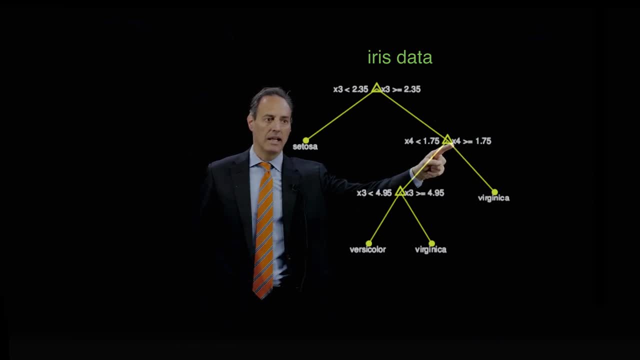 to 1.75 is virginica, And then if it's less than 1.75, I come down here to the third split, And at 4.95, I go to versicolor or virginica. So virginica lives on these two balls, which was those two? 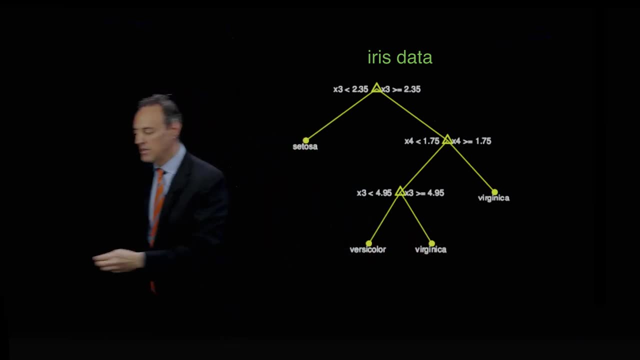 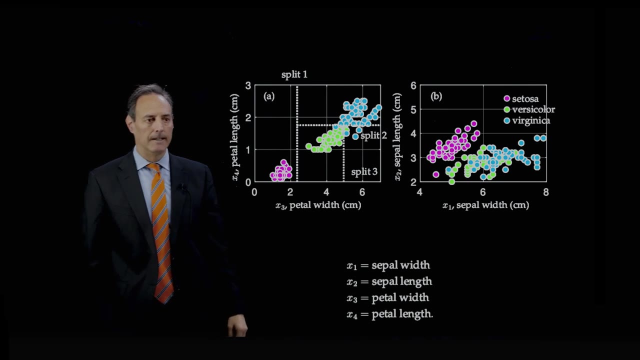 boxes. Versicolor is here, Cytosis is over here. Notice that everything is a nice, simple parallel cut In the data. Okay, So that's a nice way to do it. There are other techniques, innovations around this which allow you to do other kind of cuts, but this is one. This is the standard way to think. 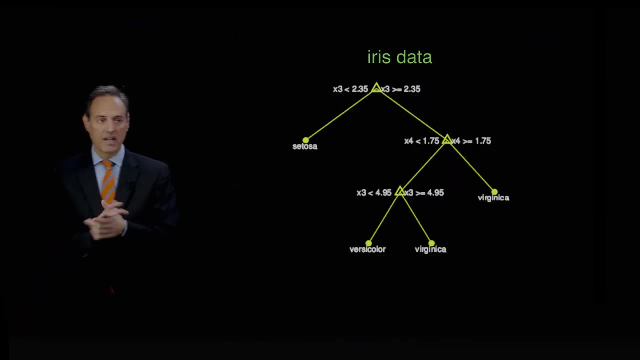 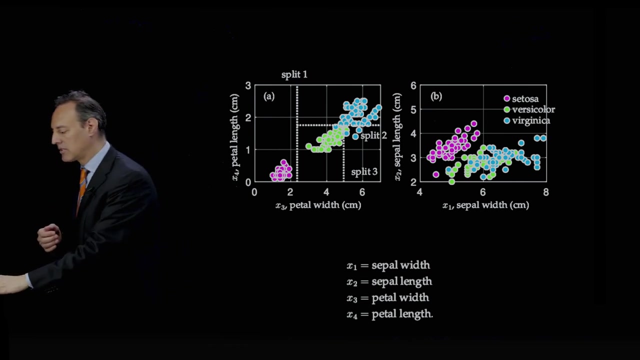 about the decision tree and the cutting. So that's the iris data, That's its decision tree. Pretty nice, right? Very interpretable. I mean you can start looking at these X3, remember the interpretation being here that X3 is the petal width. So if the petal width right, so that's. 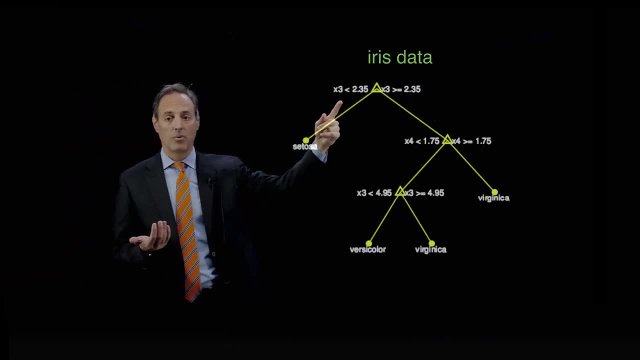 you can go back here and say if the petal width is less than 2.35 inches or greater than 2.35 inches. I know that if it's less than 2.35 inches it's a cytosis, Or I'm going to classify it as a. 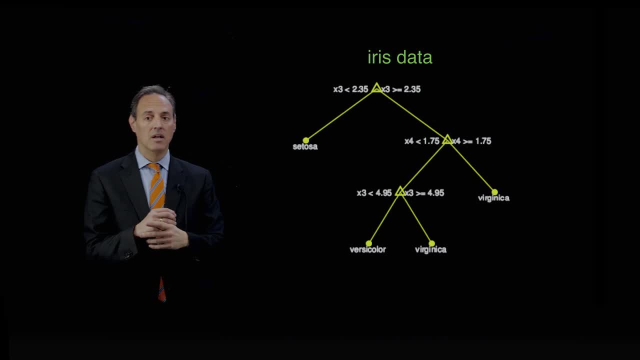 cytosis. So it's starting to give you very interesting information and interpretable information. So decision trees are actually really practical and important because oftentimes what they pull out for you is meaningful information that you can actually understand, interpret and make decisions. 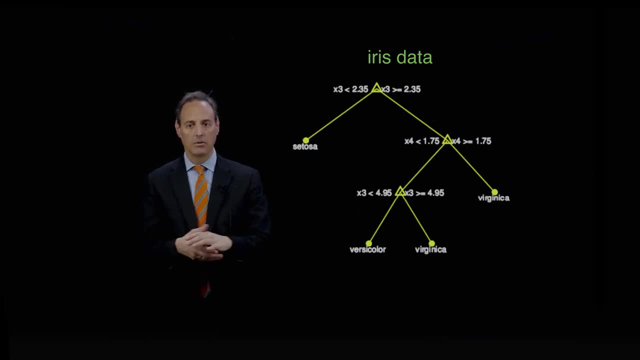 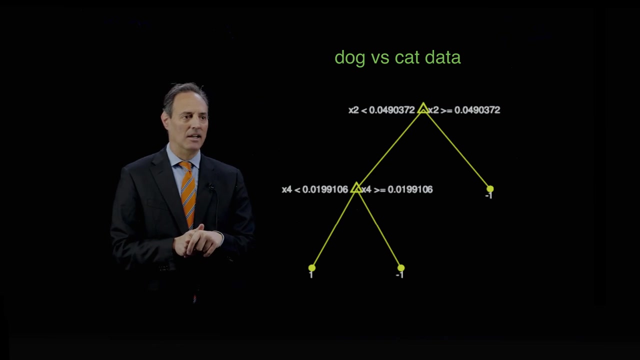 Okay, So that's why they were so commonly used, in addition to the fact that they're easy to execute And you can go to high dimensional data and do this very nicely. Okay, here's the dog versus cat example. Same kind of thing We can split along the two major directions, X2 and X4.. Those are: 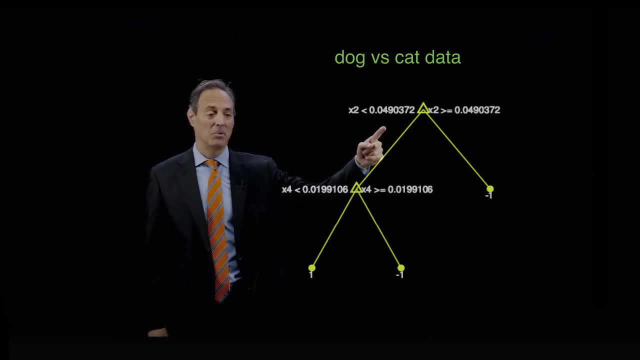 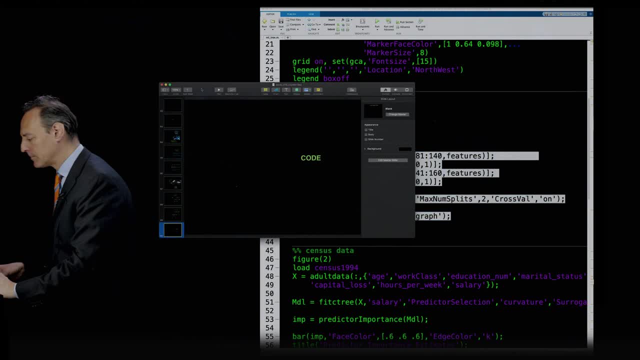 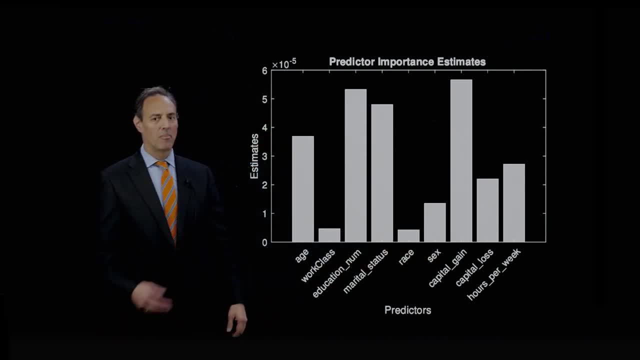 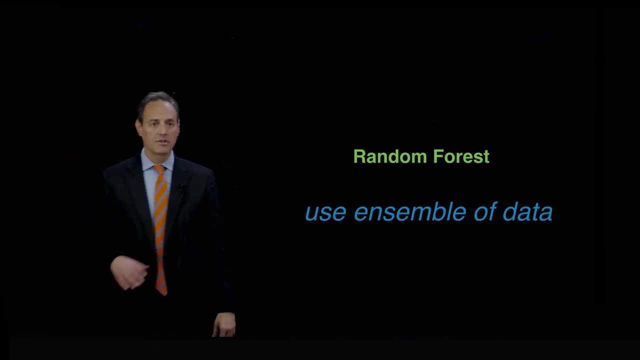 Now, before I finish on this, I do want to mention one important thing, which is this idea of random forest. Okay, So, every time you do this with sort of either noisy data or very high dimensional data, whatever training data set you pull out to sort of build these trees with, the training set itself can actually dictate very different tree structures. 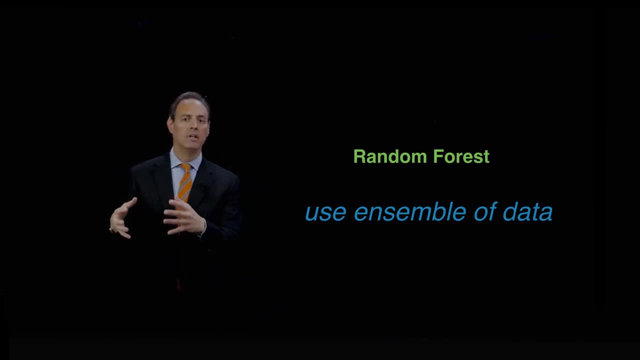 If I randomly pulled a different training data set, I'd get very different decision trees, So this is a little bit problematic. In the last lecture, support vector machines- I showed you that if you cross-validate dog-cat data, you can get models that are amazing and models that are not very good. 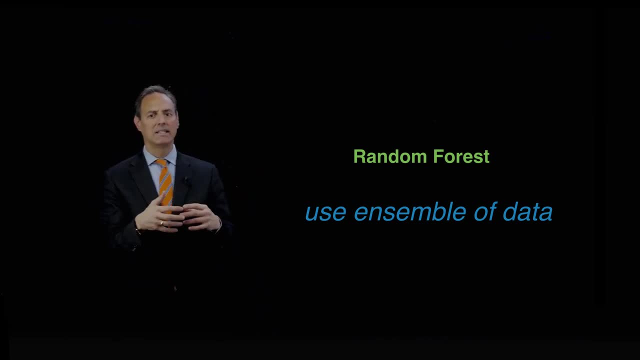 So you have to cross-validate. So random forest is in some sense an attempt to cross-validate And the idea here is to use ensembles of data. It's very much looking like a K-fold validation. You do random draws of the data to build different trees. 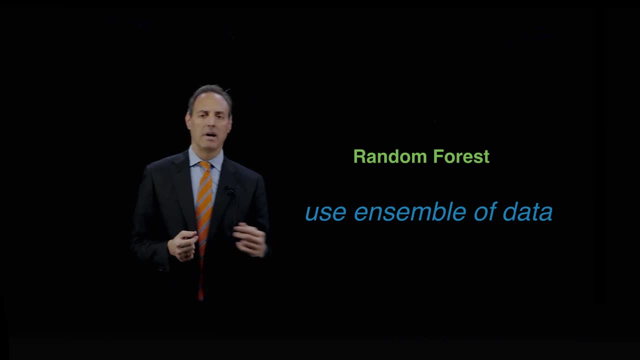 And you use the average of those models, or an ensemble of those models, to actually do your prediction Right. So you don't rely on one training set which essentially produces its own bespoke classification tree, while another training set would produce a different classification tree.